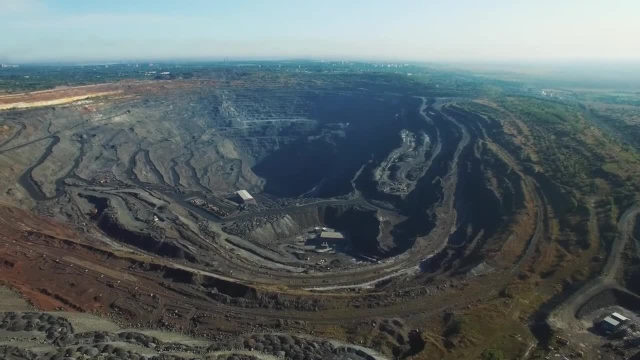 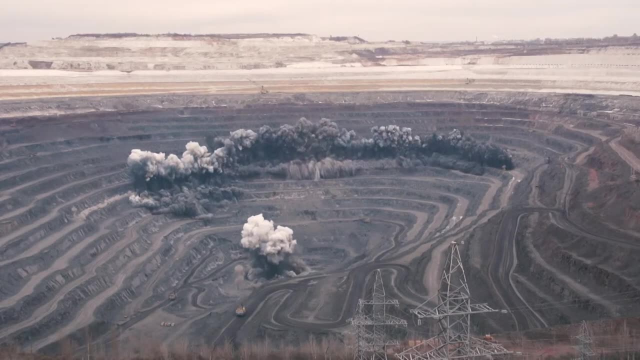 Coal is a fossil fuel that is found beneath the surface of the earth. To get coal, a mine needs to be constructed. To make coal, a mine must be constructed by drilling into a hole. This can cause large and wide scale changes to the environment. 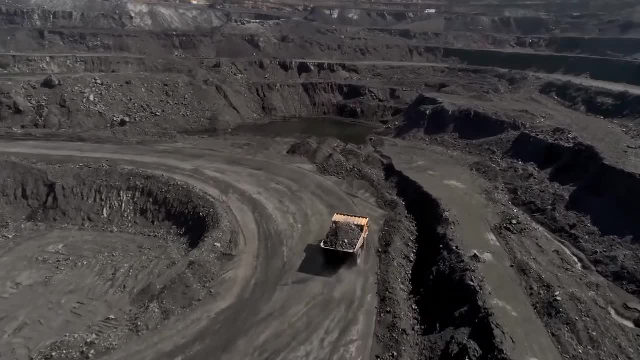 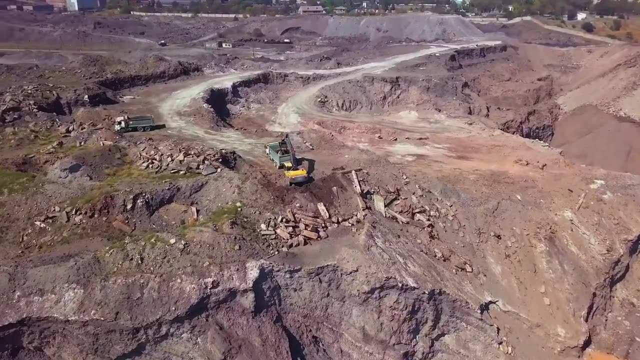 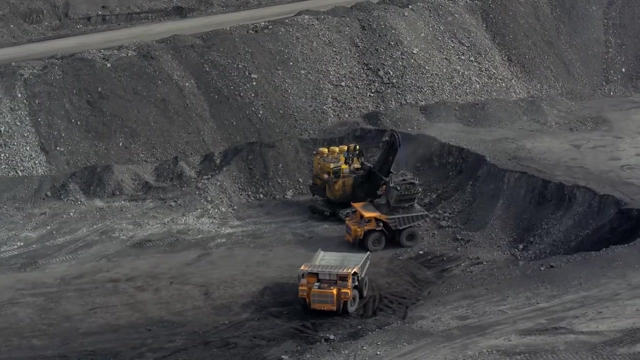 Trees and plants are removed to make way for the mine and the network of roads needed to transport people and coal out of the mine. A major impact of coal mining is habitat loss. This occurs when human changes to the environment result in there being insufficient resources. 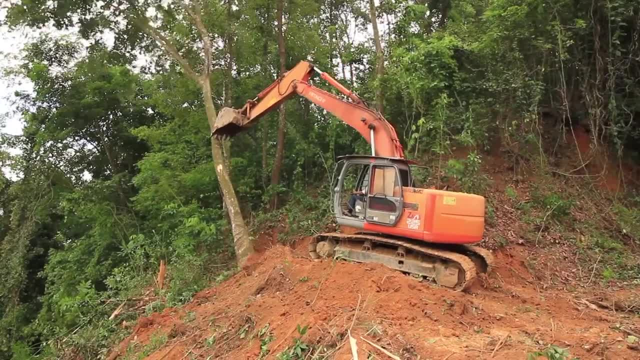 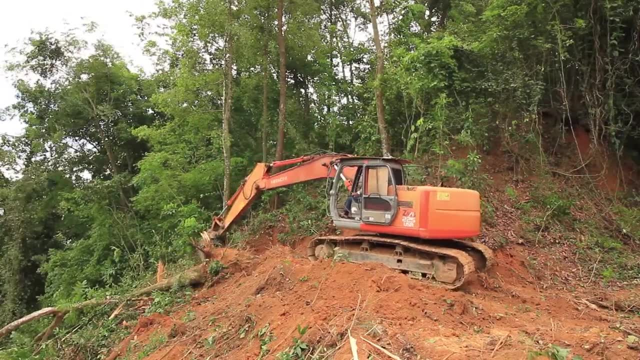 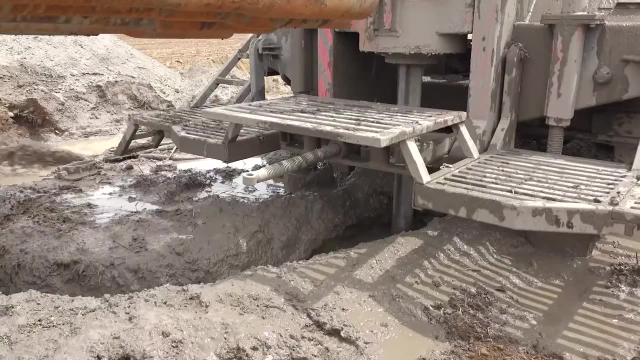 for organisms to survive, Some animals may move to a new, suitable habitat. Most organisms, however, will die. To get natural gas and petroleum, people must drill deep into the earth's surface. Sometimes chemicals are used to pump the fuels from the earth. 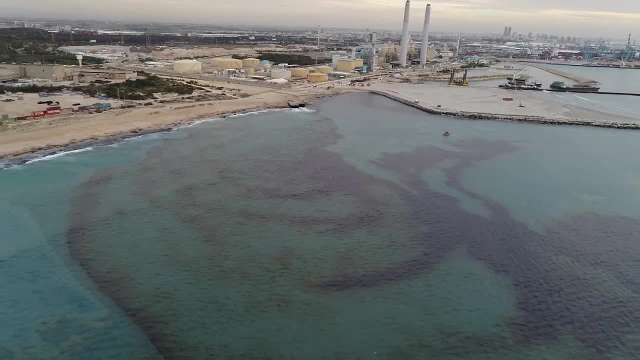 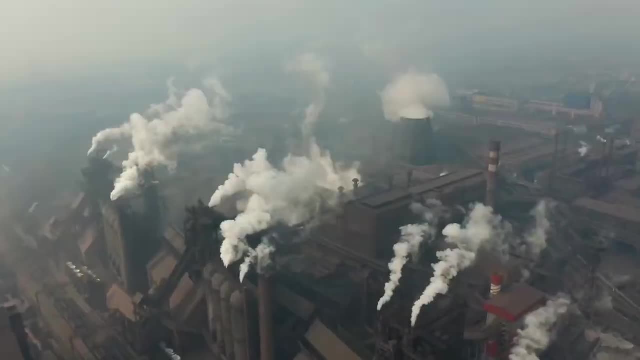 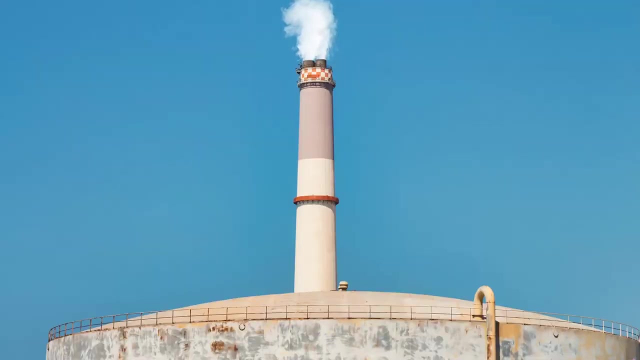 These chemicals can pollute the land, Land and water. pollution can also occur when the fossil fuels spill into the natural environment. The burning of fossil fuels has another impact on the earth: air pollution. The emissions released into the air when fossil fuels are burned are harmful to organisms. 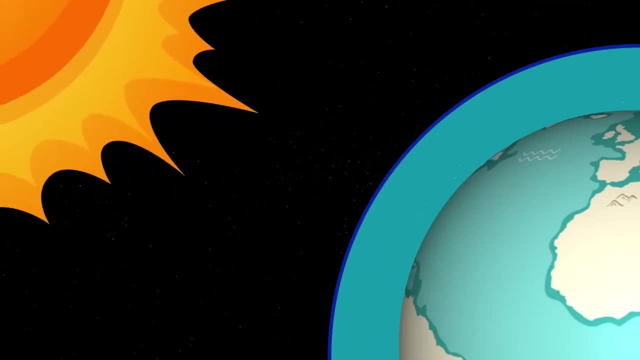 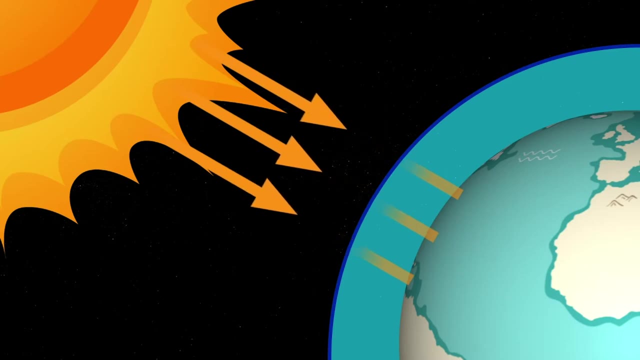 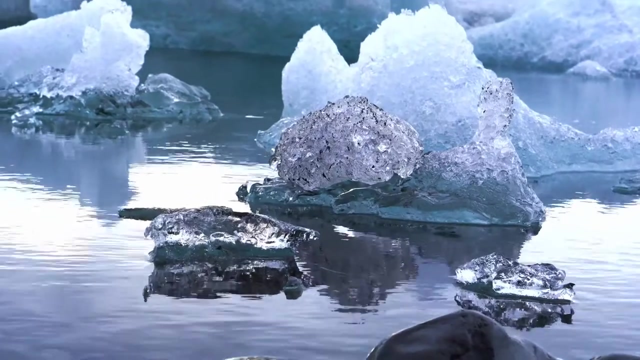 including people. The emissions also include greenhouse gases that trap solar radiation in the atmosphere and increase the rate at which the earth is warming, a process called human-induced climate change. Scientists have discovered so much more than just fossil fuels, With solid evidence that the burning of fossil fuels by people is causing the earth to get. 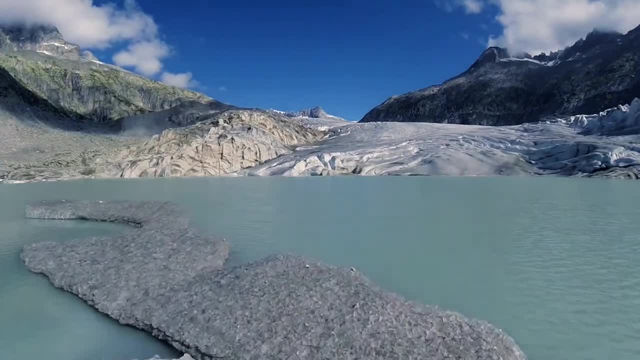 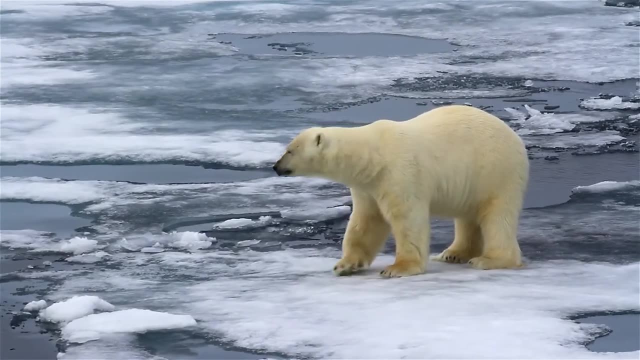 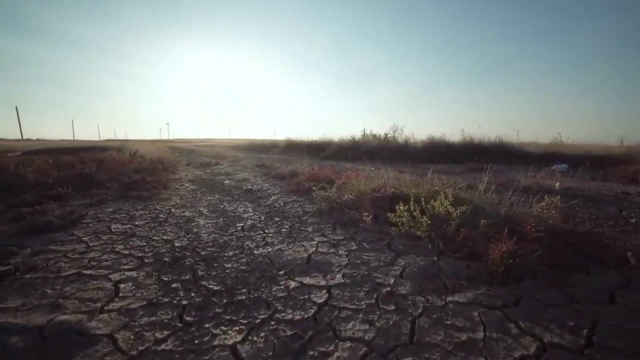 warmer at a much faster rate than it normally would. This has caused the water level in the oceans to rise, the melting of the earth's polar ice caps and causing changes to many of earth's habitats, making them unsuitable for the organisms that depend on them. Don't forget to subscribe.